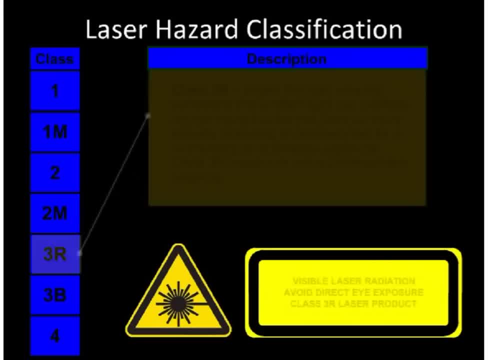 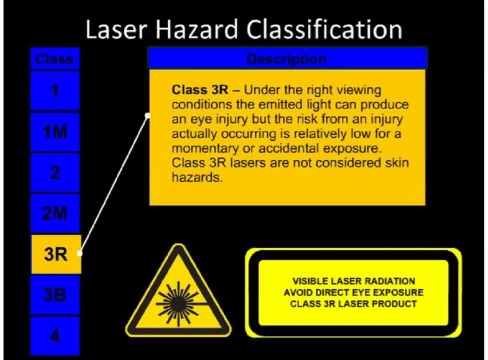 telescopes Class III R. Under the right viewing conditions, the emitted light can produce an eye injury, but the risk from an injury actually occurring is relatively low for a momentary or accidental exposure. Class III R lasers are not normally considered skin hazards. 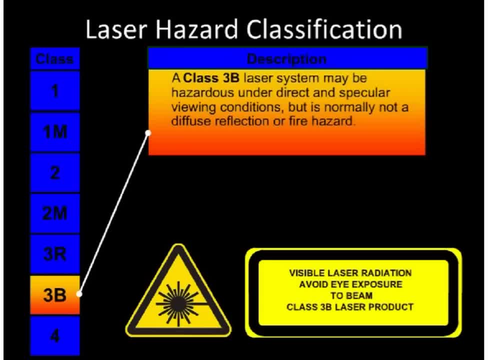 Class III B. Eye damage is likely to occur if the beam is viewed directly or reflected from a shiny, mirror-like surface. This includes an accidental or momentary exposure. If the laser emissions are near the upper limits for Class III B, the laser light might be. 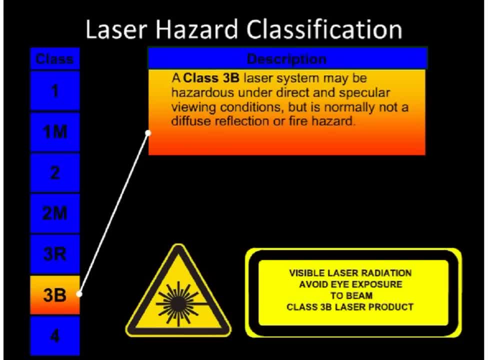 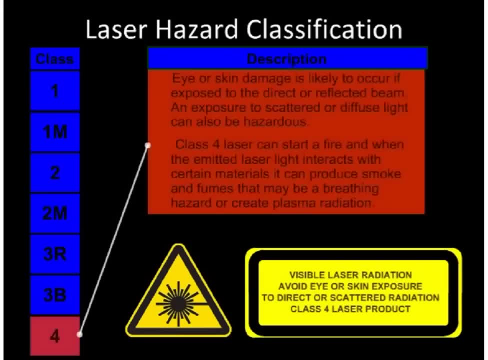 capable of producing minor skin injuries or even pose a risk of igniting flammable materials. Class IV Eye or skin damage is likely to occur if exposed to the direct or reflected beam. An exposure to scattered light can also be hampered. hazardous Class IV laser light can start fires and when the emitted laser light interacts. 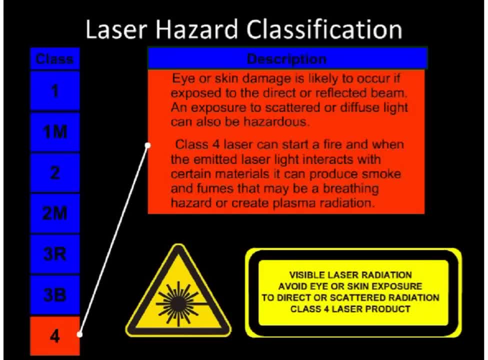 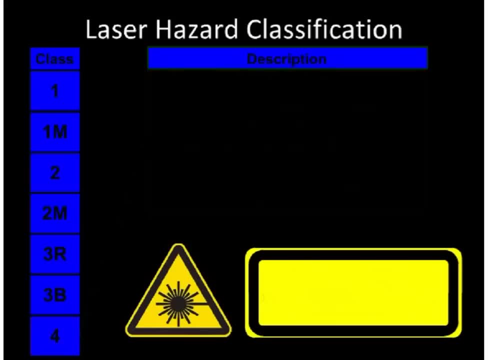 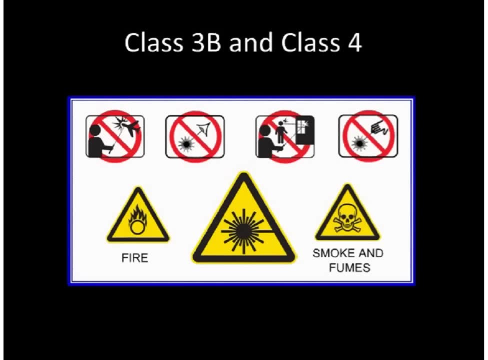 with certain materials it can produce smoke and fumes that may be a breathing hazard. In some cases it can even create plasma radiation. Class IIIb and IV lasers are the most hazardous types of lasers and require the most controls when used. Regardless of the hazard classification, almost all lasers, including Class I, that 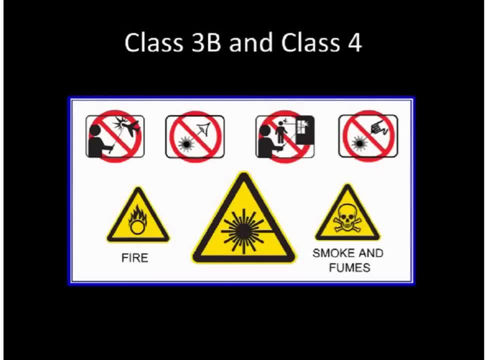 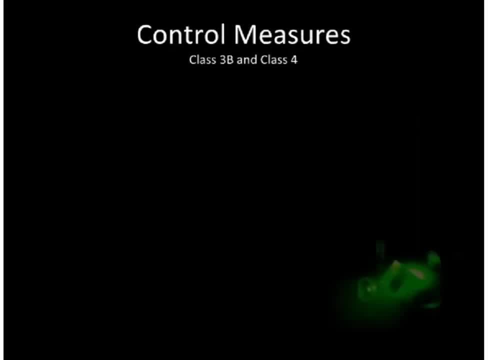 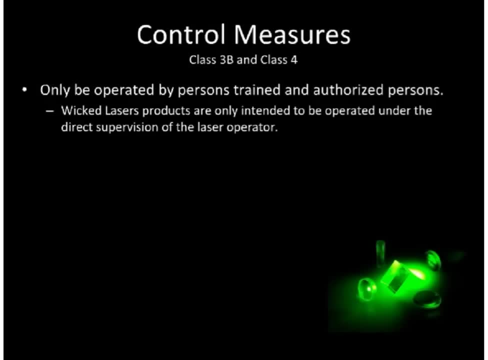 emit visible laser light can cause a distraction or temporarily impair a person's vision. under the right circumstances, At a minimum Class IIIb and IV lasers must only be operated by trained and authorized personnel. Wicked laser products are only intended to be operated under the direct supervision of the laser operator. 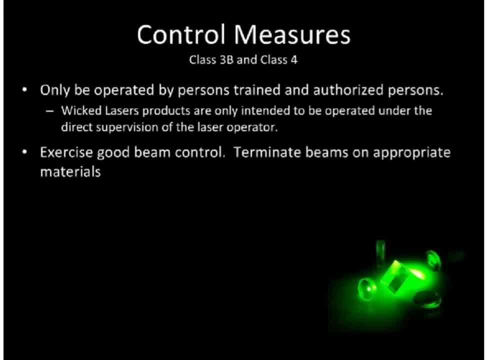 Exercise good beam control. Terminate beams on appropriate materials. Never direct the beam at persons or an aircraft. Be aware of where your beam is going. Be aware of the effect of introducing optics or other targets into the beam. Nowhere reflections might redirect the beam. 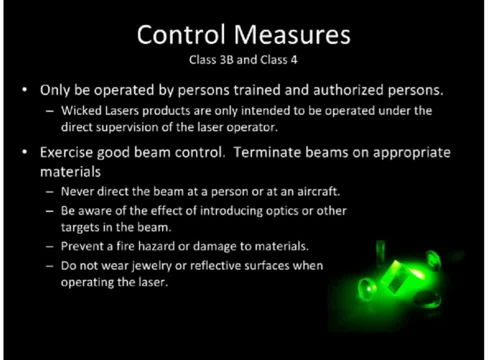 Prevent a fire hazard or damage to materials. Class IV and some Class III beams can char, burn or ignite materials. Especially avoid exposing dark, thin and combustible materials. Do not wear jewelry or reflective surfaces when operating the laser. Enclose the emitting laser energy as much as possible. 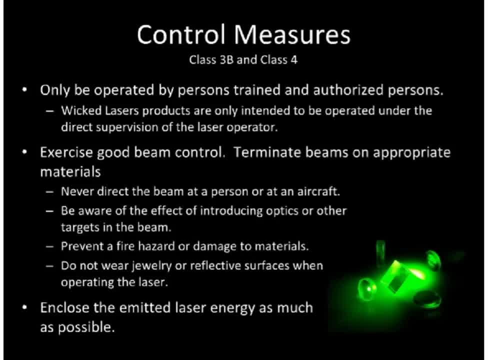 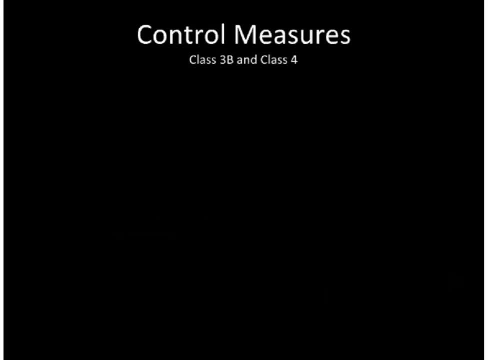 Exposures need to be made up of materials that will not transmit levels of laser light above the maximum permissible exposure or be subject to damage from the anticipated laser exposure. Establish a laser-controlled area. This area should contain the nominal hazard zone. Anyone occupying this area while the laser is operated must be protected from all laser. 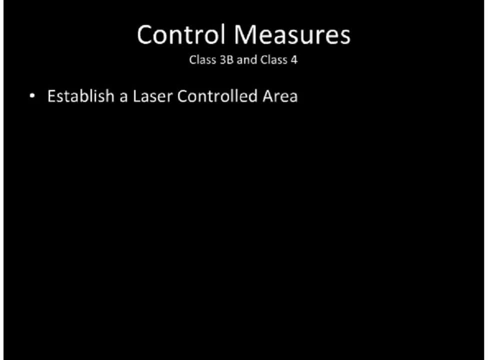 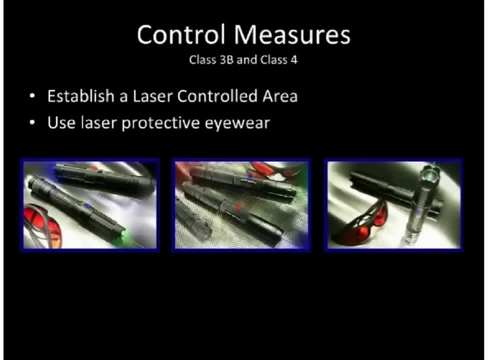 hazards. All unnecessary personnel should be located outside the controlled area when the laser is operational. Laser protective eyewear should be worn by anyone in the laser-controlled area when Class 3B lasers are operated and must be worn by persons within the laser-controlled area when. 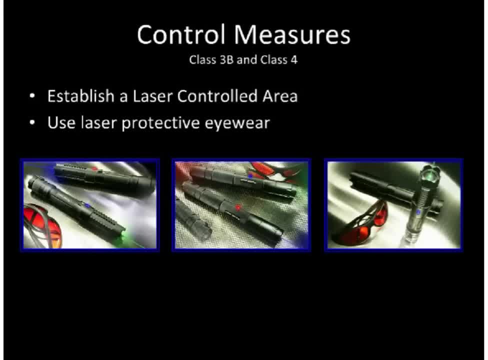 Class 4 lasers are operated. Wicked Lasers provides laser protective eyewear rated for the use with specific models of their Class 4 laser products. Eyewear must be labeled with the protection it provides. Different countries have different requirements. You should contact a laser safety eyewear provider that is familiar with the laser safety. 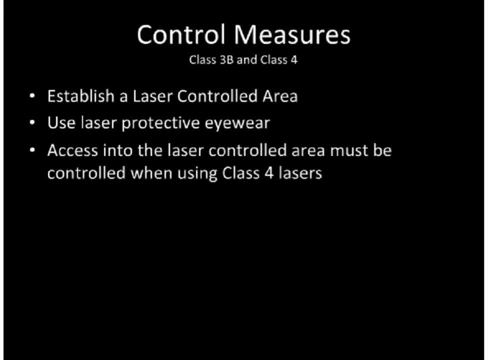 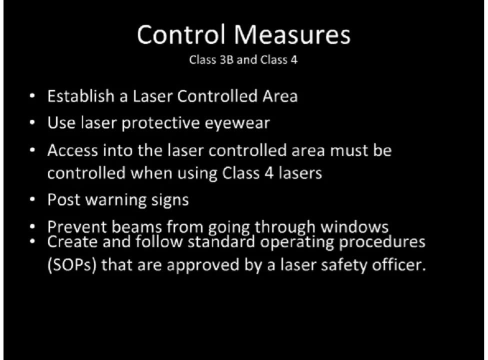 requirements in your location for additional details. When using Class 4 lasers, access into the laser-controlled area should be controlled. Post warning signs at the entrance to laser-controlled areas. Prevent the possibility of the beam going through a window. Create and follow standard operating procedures that are approved by a laser safety officer. 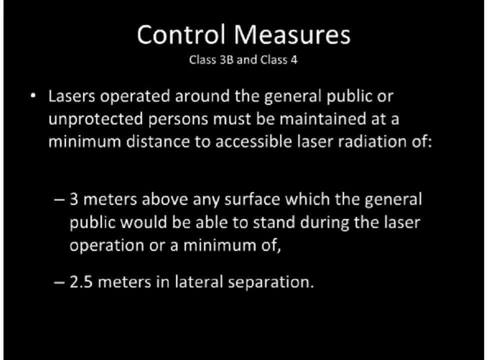 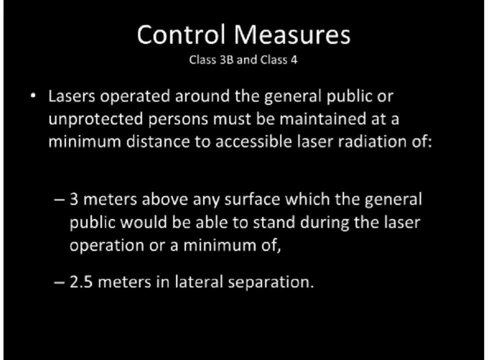 All laser safety eyewear must be maintained. All laser safety eyewear must be maintained at a minimum distance to accessible laser radiation of three meters above any surface which the general public would be able to stand during the laser operation, or a minimum of 2.5 meters in lateral separation. 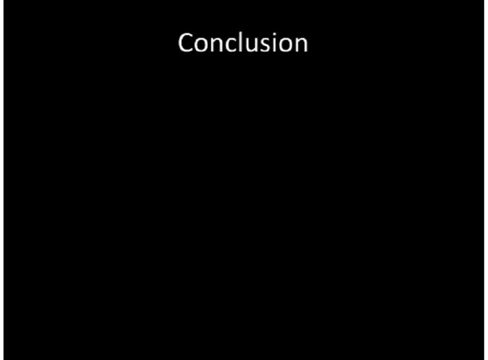 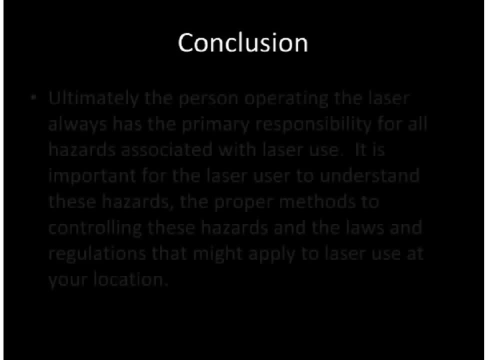 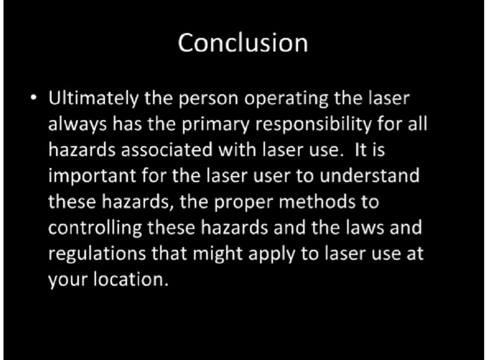 This presentation only covers basic laser safety topics at an introductory level. It cannot cover every topic in the detail necessary for your specific laser use. Ultimately, the person operating the laser always has the primary responsibility for all hazards. It is important for the laser user to understand these hazards, the proper methods to controlling. 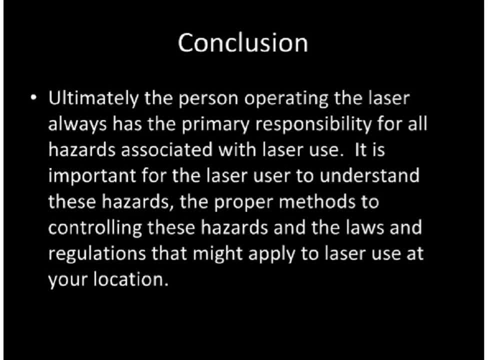 these hazards and the laws and regulations that might apply to the laser use at their location.